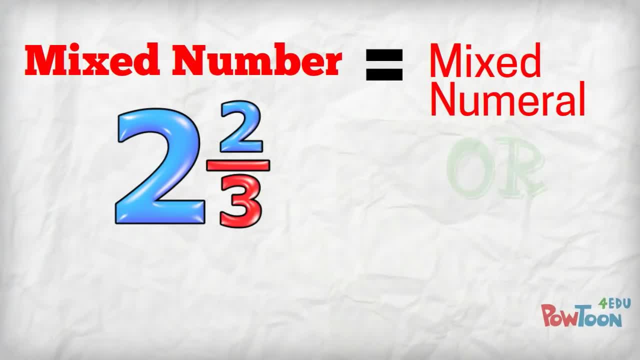 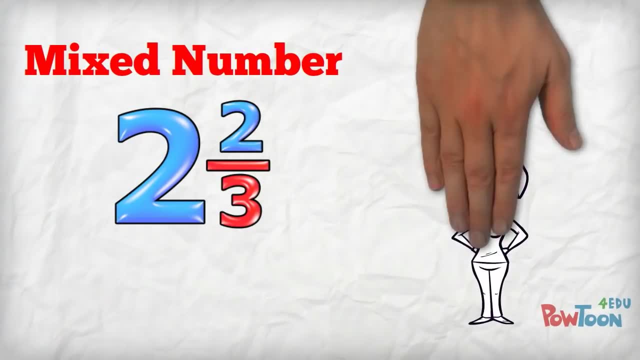 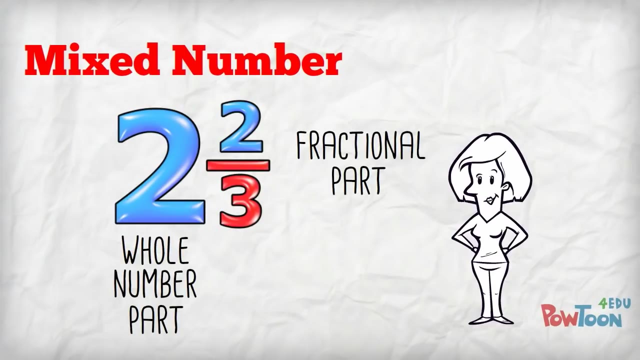 You might also hear this thing called a mixed numeral or a mixed fraction- Different names, but they all mean the same thing. Every mixed number contains a whole number part and a fractional part. Here we've got 2 and 2 thirds, that's 2 whole ones. 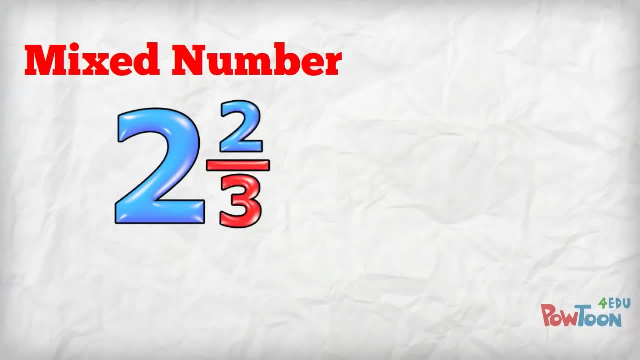 and the fractional part is 2 thirds. When we change between a mixed number and an improper fraction, we're saying how many parts there are in total, and we're giving that information in the form of a fraction. The denominator tells us how many parts are in each whole. 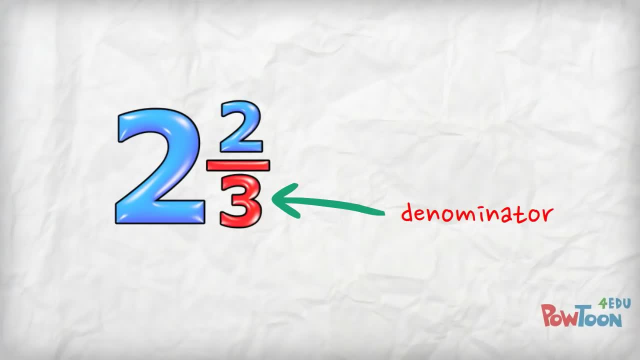 A denominator of 3 means that each whole has 3 parts and we have 2 wholes. This fractional part tells us that we have 2 parts out of 3.. We can see all our parts in this diagram. How many parts have we got? 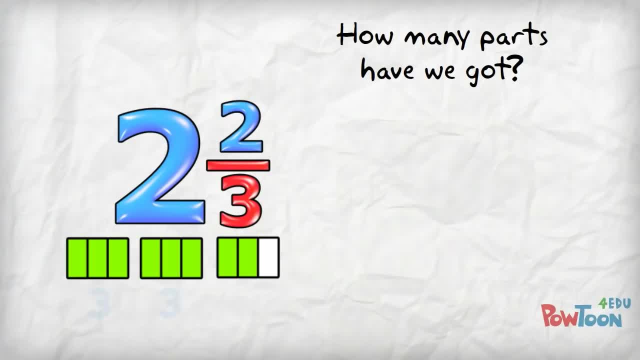 There are 2 wholes, so that's 2, lots of 3, 6 plus 2 more parts, that's 8, and we keep the same denominator because this is still parts out of 3.. So we put the total number of parts, that's 8. 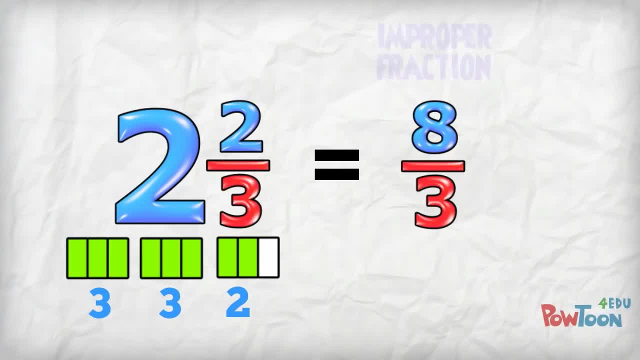 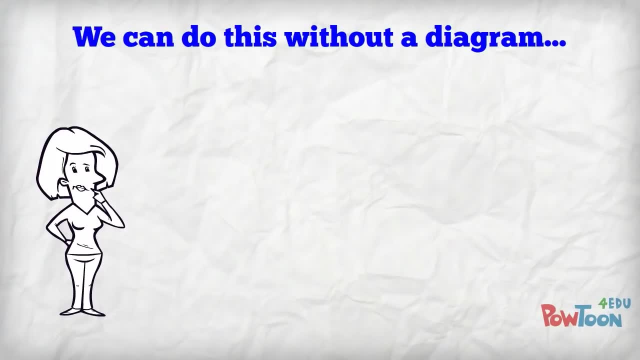 over our denominator of 3.. And there's your improper fraction. We can also do this work without using a diagram. Let's take another example: 4 and a half. Each whole is worth 2 because our denominator is 2.. I have 4 wholes. 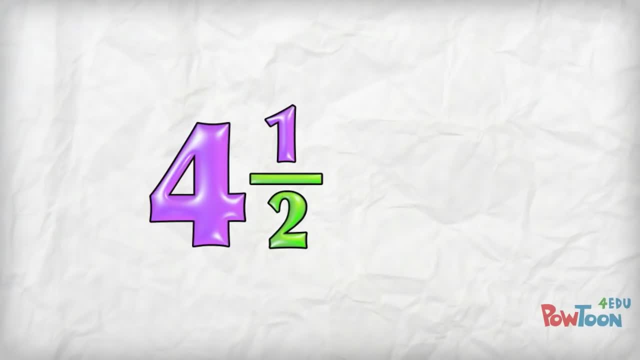 so that means I have 4 lots of 2, or 4 times 2. that's 8, and I have another part here to add in from the numerator of 1.. So 8 plus 1 is 9. That's our number of parts. 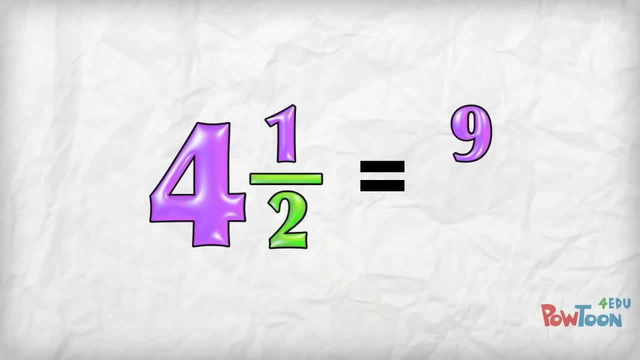 so that's our numerator. I use the same denominator. we started with 2 and I'm done. 4 and a half is the same as 9 over 2. And I can use a diagram to prove it: 4 wholes- Each whole- is worth 2 parts.